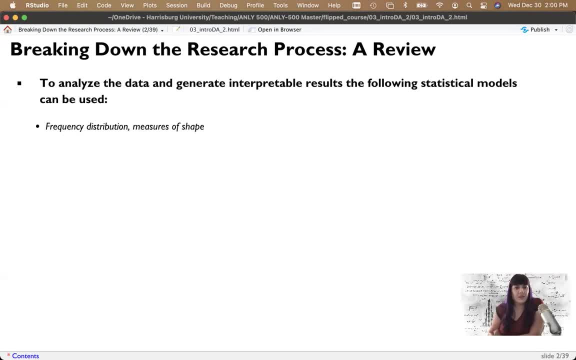 And so in this lecture what we're going to cover is frequency distributions or measures of shape, central tendencies or measures of distance, dispersions or measures of spread, and then end on some alternative options like a z-score, which is a bit of a measure of of a distance, and association, which is correlation. Now we have a whole separate. 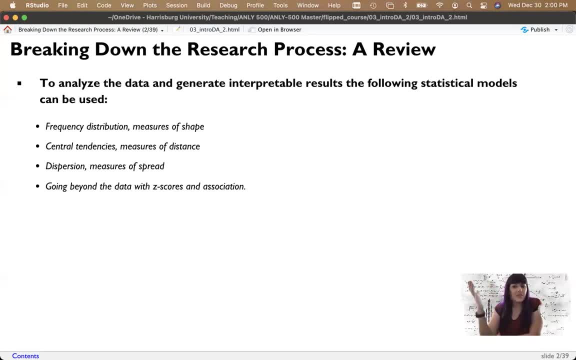 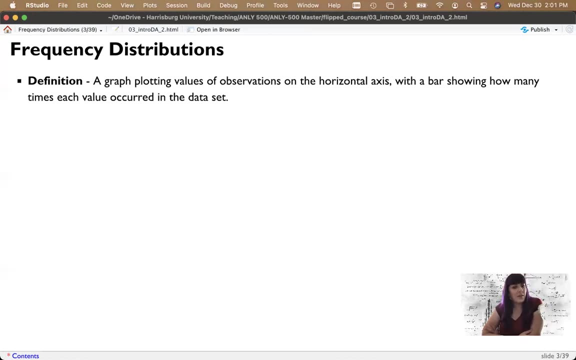 week on correlation, but you can get the basic idea of like why this is a good descriptive statistic as well as a statistical test. All right, so that's our outline. Let's jump right in. So a frequency distribution is usually considered a graph, although we can also make a frequency table that plots our values along the bottom. 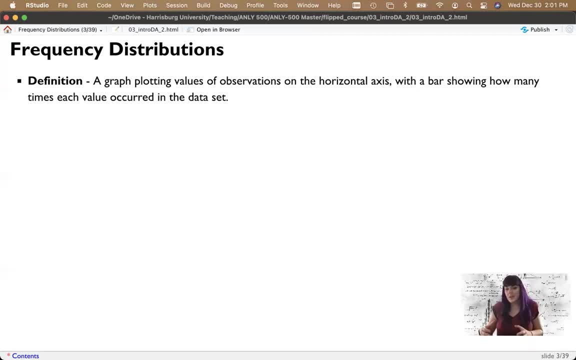 Now these values could be categorical. they could be likert, likert, they can be interval, but generally frequency distributions are held for continuous data, as more common to use them, and a frequency table, more common for categorical data, although you can make what's called a Pareto. 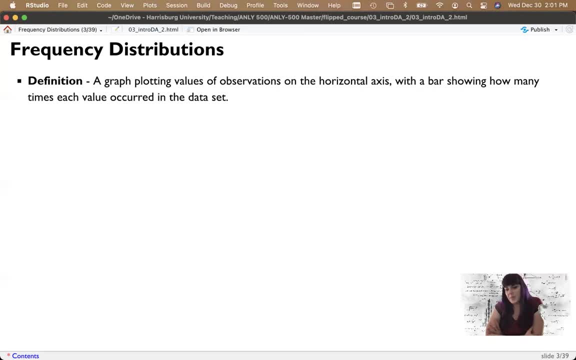 chart, which is a frequency distribution for categorical data. that puts them in like highest to lowest format, And so that's on the x-axis and then it has bars showing the frequency, or how many times, as the y-axis. So these are really good to just get a view of the distribution of the data. 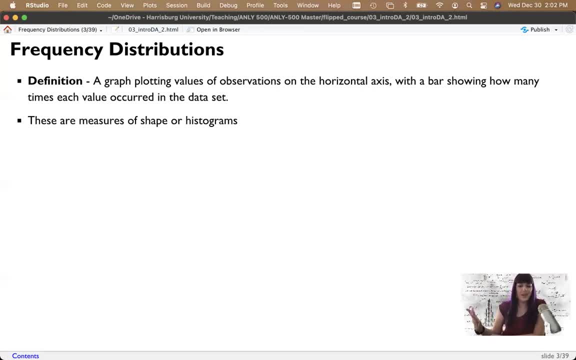 And these are measures of shape. Sometimes they're just called histograms instead of a frequency distribution, but those mean the same thing. So here's a cute little example of the normal distribution. but understanding any distribution of data can is pretty critical and we'll get into this more when we do data screening and data. 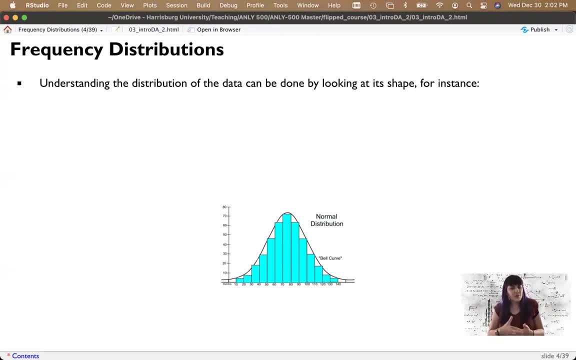 data assumptions, because many of the analyses we're going to do have the assumption of normality, for example, And so we want to know what the data looks like. Now the assumption- normality- is not actually on the data- small point there- but understanding what the data looks like. 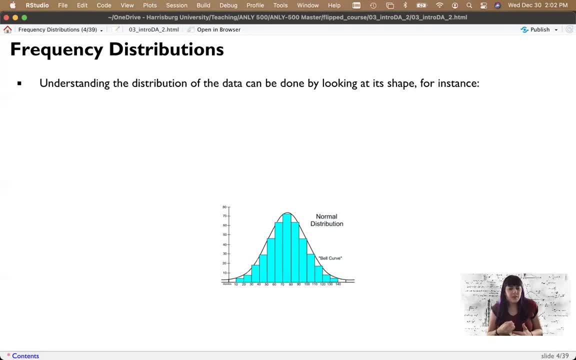 We'll help us understand outliers, so data points that are way outside the normal range, And then just skew, which we're about to get to. So it's always good to make a nice plot of your data And so we're mostly going to focus on this normal distribution. It's normal in quotes because most 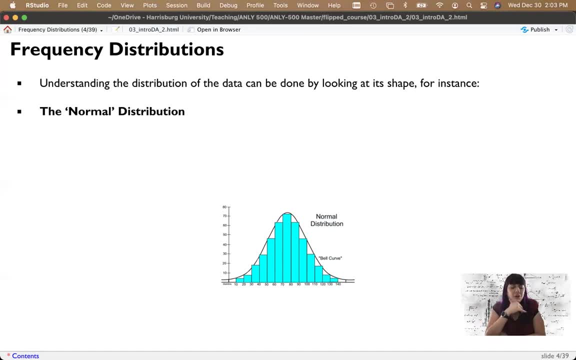 real data doesn't really fall isn't normal, right? So we talked about teaching evaluations and we're going to talk a little bit more about that in just a second. So we're going to talk about one of our last lectures and those are definitely not normal. okay, They tend to skew towards the high. 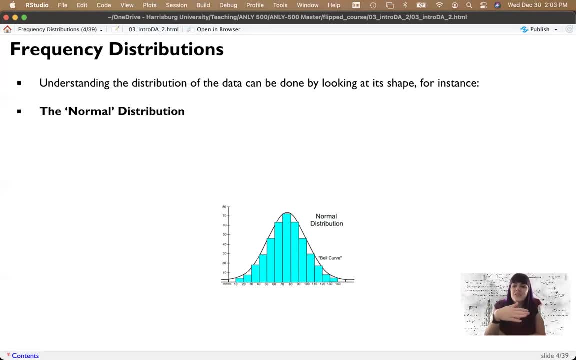 end it's really great, or towards the low end it's really bad, And so. but to describe what we mean by skew, we have to have some base comparison point. So that comparison point tends to be the normal distribution. Now there are a lot of other distributions, So there's gamma, there's beta. 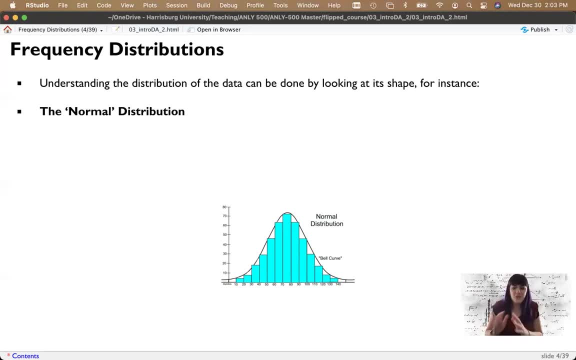 there's binomial and there's f and there's chi-square, and I could keep going. So there's so many, And they're all interrelated to each other because they can be transformed from one to another often, But let's use the normal distribution as our like comparison for understanding what data looks like. 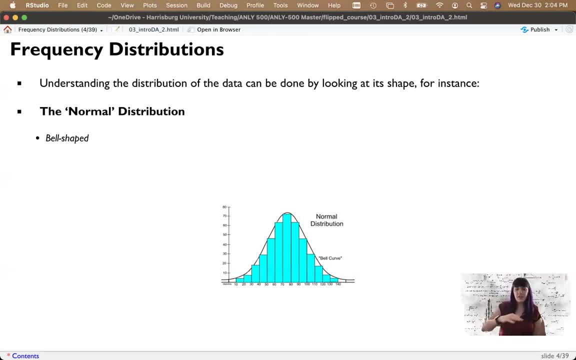 So the normal distribution itself is bell-shaped, okay, Meaning that it's even on each side. You could fold it in half, hot dog style, and the two tops would line up, okay, And so that means that it's symmetric around the center. Now, the nice thing about these distributions, when they fall. 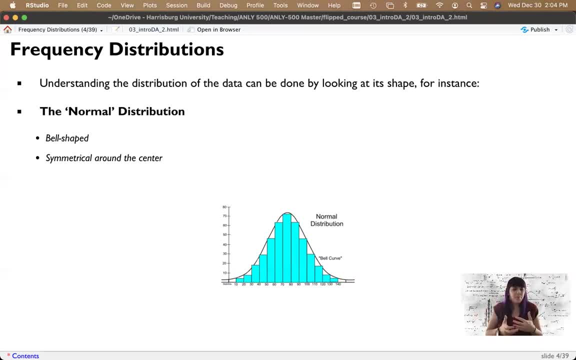 into sort of a known category. we know the proportion of the amount of data that should fall into each section. So the normal distribution here has this kind of like tall middle point And we know that- approximately 64 percent. I had to think about my table there for a second. 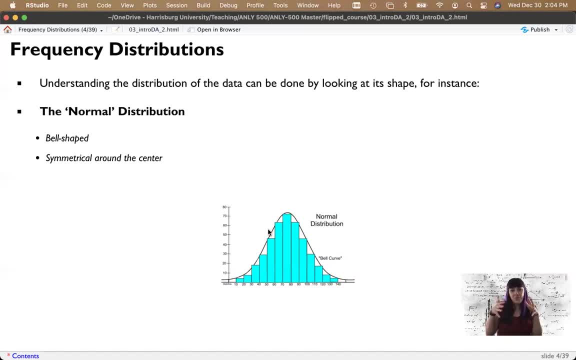 of the data should fall within very close to the mean over the middle here, And so the nice thing about these known distributions is that we can use them to calculate probabilities, which is a section that we'll get to in the next week's lecture. 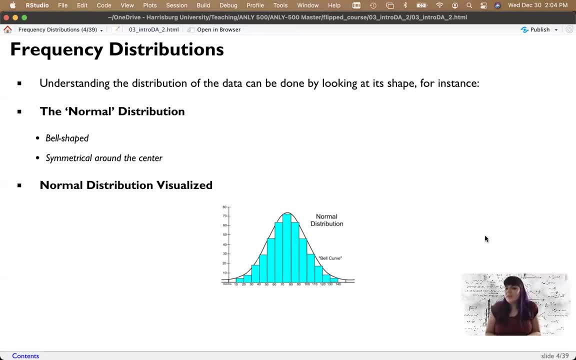 And so this is what a normal distribution looks like. Now I would say that you know, this is like the perfect normal distribution. Real data doesn't necessarily fall this way, but there are things that we can do to kind of Assume that the data is close enough right. 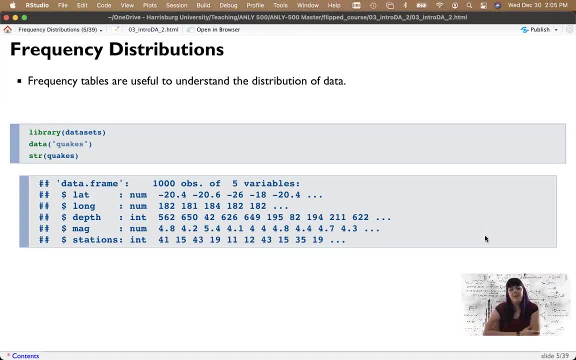 Now, a frequency table is also useful And I would say frequency tables are usually a little bit better for categorical data, So things that have labels, like we talked about in the last class, binary, nominal or maybe even ordinal data, Whereas the graph, the histogram, is usually a 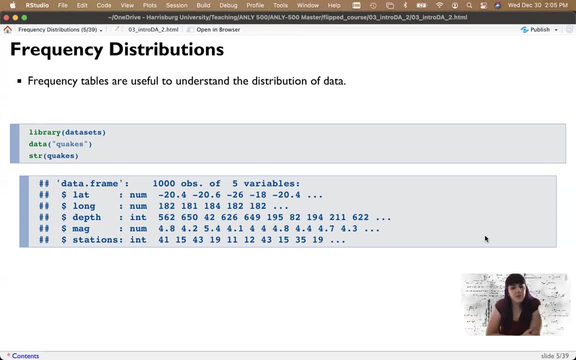 little bit better for conceptualizing that kind of thing- continuous level data- but it's really easy to make a frequency table. So let's look at this data set. We're going to use this quakes data set a few times here, So I loaded the data sets. 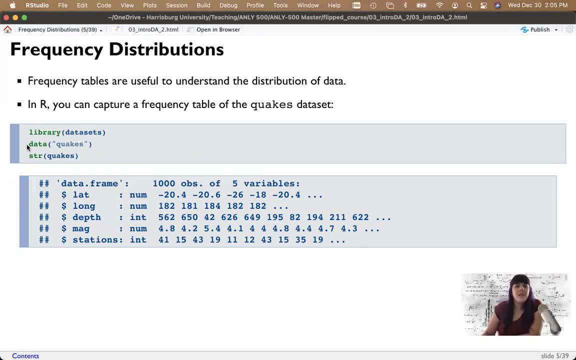 library. Don't forget, you have to turn them on when you get started. I said: you know what? give me that quakes data and let's just see what's in it. Okay, So the quakes data set has latitude and longitude of where the earthquake happened, the depth and then the magnitude of 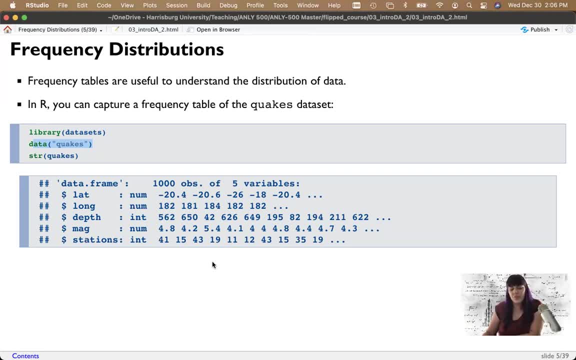 the earthquake Station. here is just which station recorded it. Okay, So while station is an integer, here it's really almost a categorical variable, in the sense that this is more of a label than it is an actual integer, Right? So let's look at the table function. 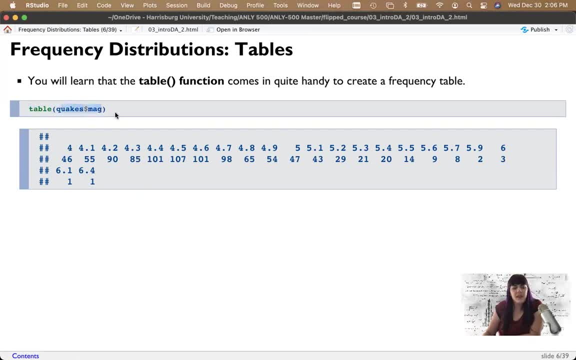 So here we have table and we want to just calculate the table of the table: Frequencies, the magnitudes of the frequencies- Wait, I said that backwards- The frequencies of the magnitudes. So the table function is really handy for that And we'll use the table function a lot when we're 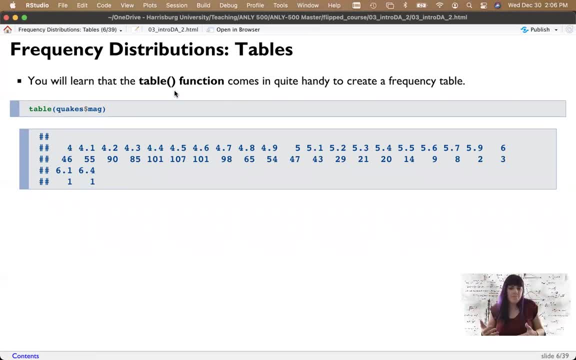 kind of testing, if data is what we think it is. So one issue that you might have with scales is they might be reverse coded. Let's have another. let's have another sip of my coffee here. Reverse coded And reverse coded scale is one where you you answer it one to five, but because of the way it's worded we flip that score so that it matches the rest. 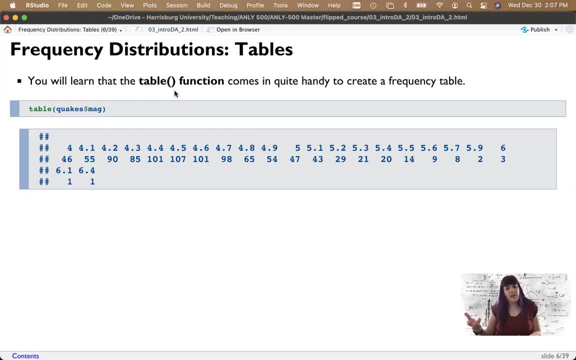 of the scale, And one thing I like to do when I'm working with these is just create a frequency table using the table function here of the like one to five, do my reverse coding and then just make sure that that table is then just flipped over. 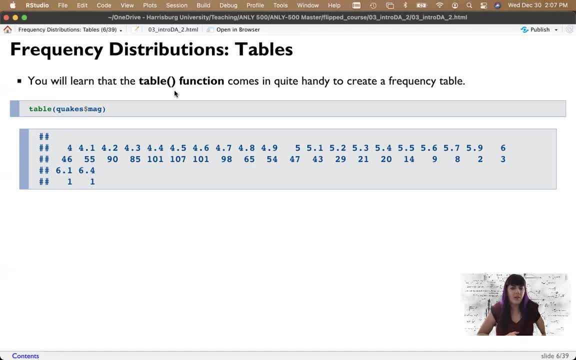 So the reverse coded tab takes those two numbers, So they're really handy for more than for, like, just checking. make sure you're doing stuff right when you're practicing coding. So what do you put in the table function? Well, the main argument is some vector of data. Okay, don't do table on an entire data frame. It actually, I think, will warn. 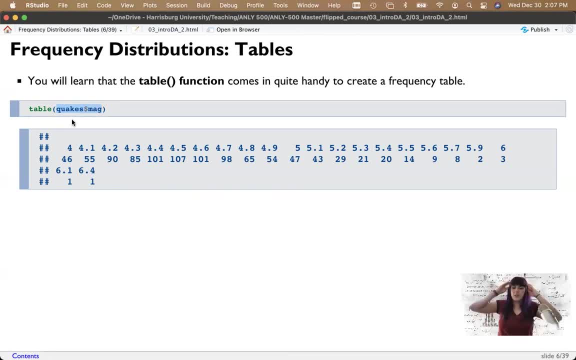 you that this is a very bad idea. So tables can be on one vector or several vectors and it'll create what's called a conditional frequency table based on if you have two of them right it'll base, you know, all the values of one by all the values of the other Makes a really big chart. So I wanted. 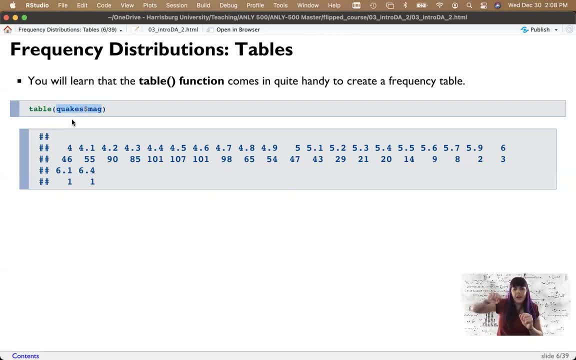 to look at gender and handedness, for example, I could have identify as male or female and then left and right hand, and so I get a little two by two table of the frequencies. So that's conditional because there's more than one variable. So just be careful doing those, because if you tell it to 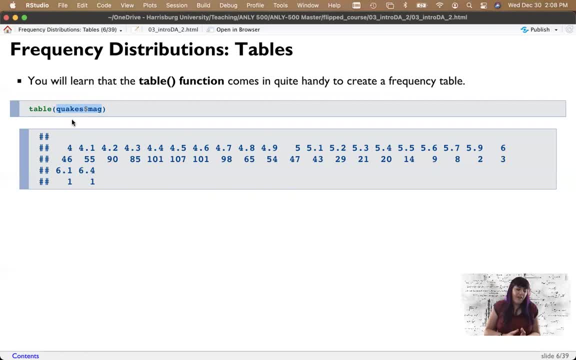 make a table. it's going to be more than one variable. So if you tell it to make a table- I have totally done this and crashed R on the entire data frame- It tries to do every variable conditionalized on the other ones and if you have 400 columns it gets really mad and then you have to. 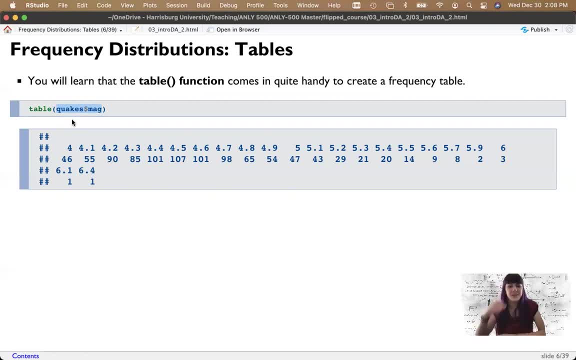 crash R studio and start over. So don't do that. Generally, what we're just going to do is put in a vector here. Now, what do we get out of this? Well, what we get out of it here is the first or the top row. Now, this goes on to two rows for me, but the top row here. 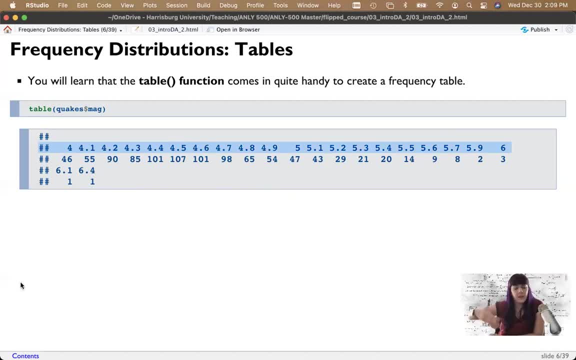 are the actions. So the first one is the number of numbers, because they're actually values in the data. Okay, so we've got earthquake magnitude starting at four here, going up through 6.4.. Now those are the actual data values in the data. The second number, the bottom number here, is the. 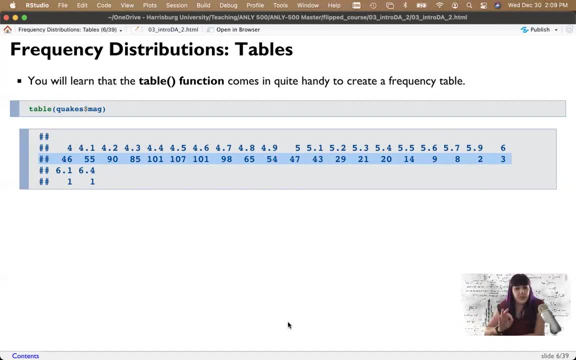 frequency of those values. So that's why a table can be really tedious for continuous data, because if you have data with lots of decimals it just gets really long table data. that is one thing or this or that right. so for factors as in the table, small, but here we're. 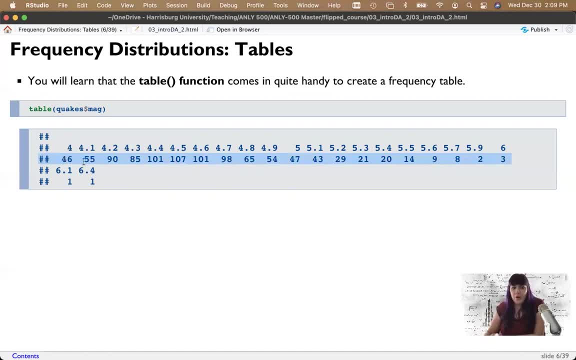 sort of somewhere in the middle. so we have 46 earthquakes that were a four um, 55 earthquakes that were 4.1 and up. now i can kind of look at this data and see that there are some bigger numbers here towards the bottom of the scale. so maybe it's not normal because we might expect the biggest. 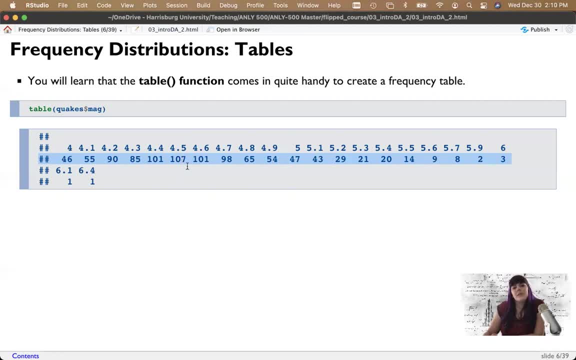 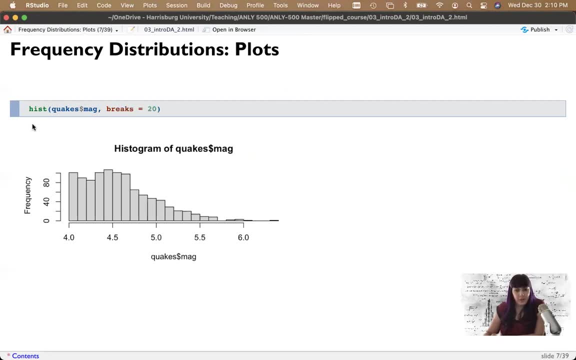 numbers to be in the middle of the scale. but you know this can be much easier with a picture, so let's look at that plot. there are lots of ways to make a histogram in r, but the simplest way is using the base r function. hist for histogram- histogram can take a couple arguments, but here's. 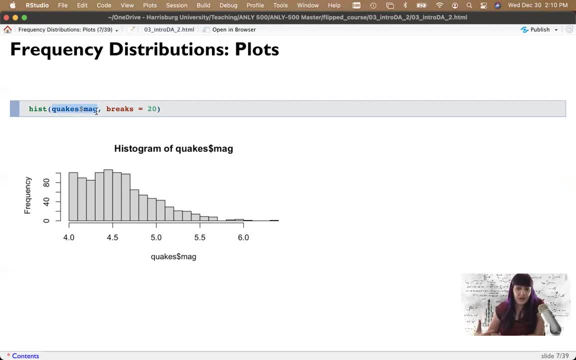 the main two. so the first argument is the vector of data that you want to put in. so we put in our quakes column, our magnitude column, and then this breaks. function is just allows you to change the, the, how big those bars are. so i'm going to flip back over to r here to show you the difference of what happens. 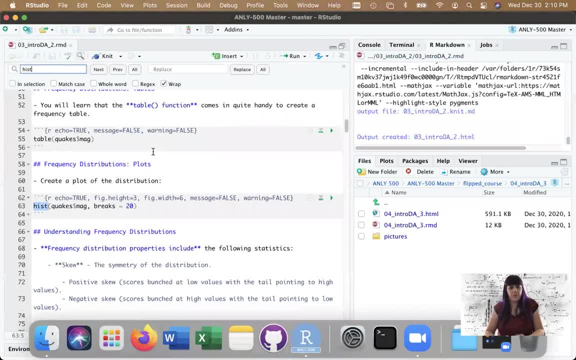 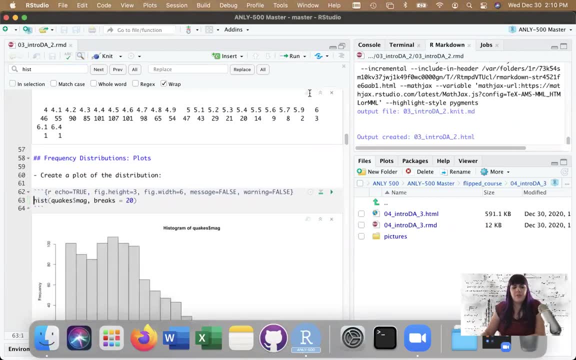 so let's go down here to histogram. it's going to tell everything above that to run. so make sure i have my data set open and then run. this breaks function. okay, so let's see if we happen. we make this one. what do you think is going to happen? 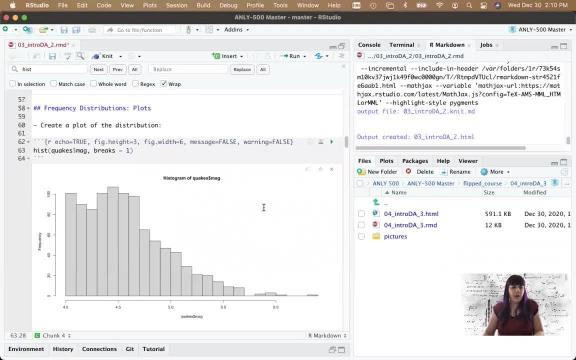 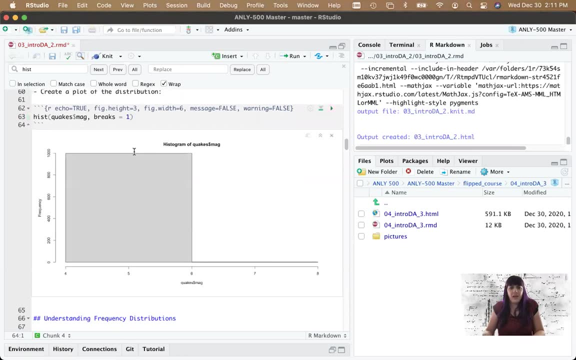 well, it's tempting to think of breaks, as how wide the window is. that's not quite how it works, right? so if i have the scale, that's four, five and six, effectively, and you make a break one, you think it might give me everything from four to five and everything. 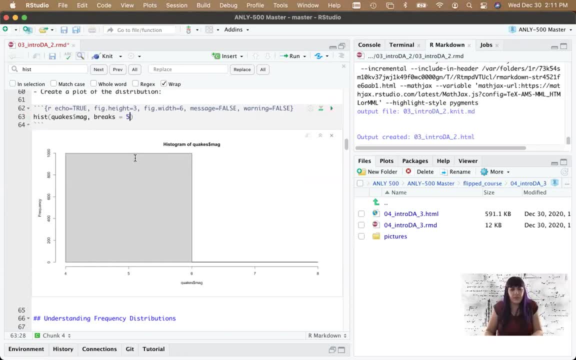 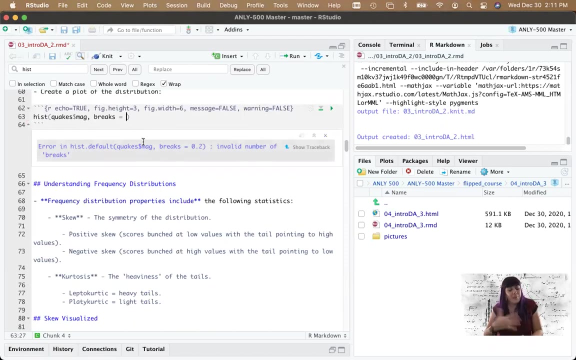 from five to six. that's not quite what i did, okay. well, let's make it five, see what happens. okay, let's make it point two. so i i have never been very it's like you know, no, don't do that, not allowed. if you have bigger data, you, you actually can. but let's make it 100, see what happens. 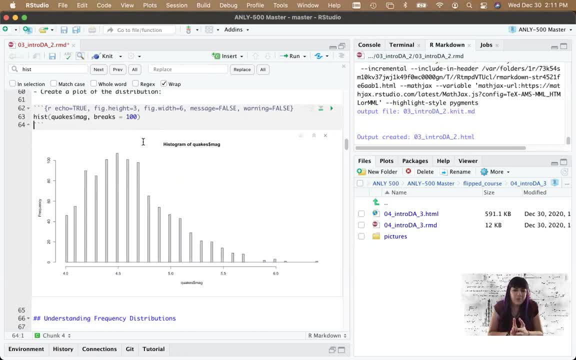 so with breaks i it always is like smaller numbers are wider windows and then, um, bigger numbers are smaller windows. you just gotta find kind of the right point. okay, there's probably some magic magic to knowing what the breaks points are, but i'm just always kind of like play with it till it looks. 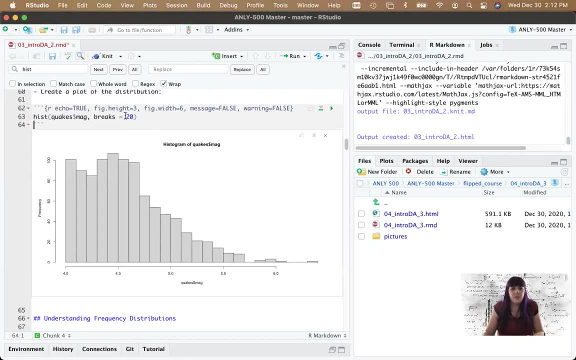 about right. okay, what do you mean by looks about right? well, you obviously don't want the bars to be really wide, because that is misleading in the data. so this looks kind of like a stair step. if i calculate breaks at about 20, i can see there's actually this dip in the data. 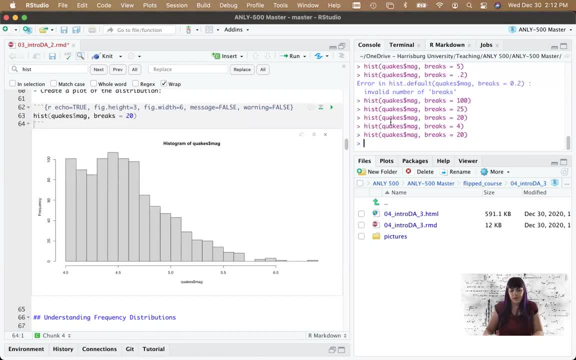 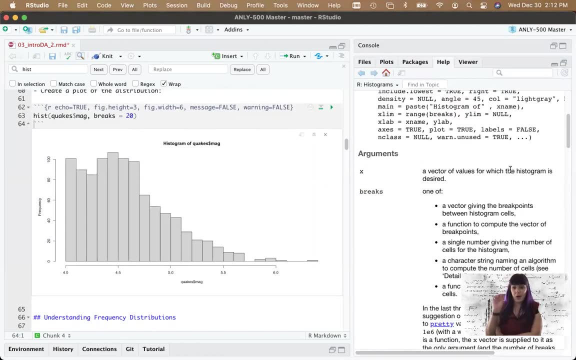 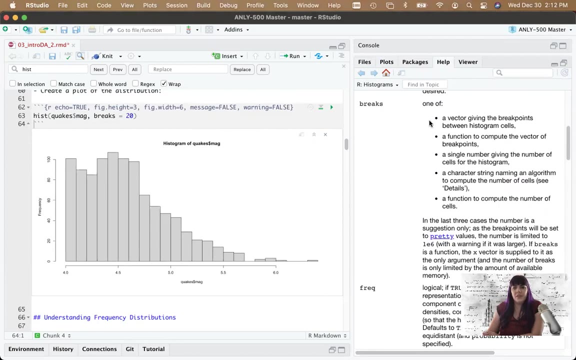 and so you're just trying your best not to misrepresent the data. let's see what it actually says that that breaks function does. maybe then i'll understand it. so let's use the help, right, so question mark hist. all right, so breaks can be a vector giving the break points. okay, so i could. 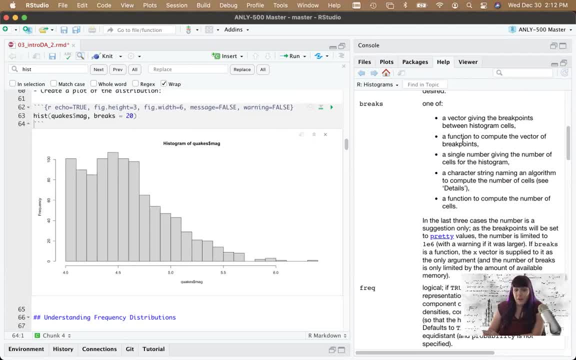 say, break at four, five, six. it could be a function, it could be a number, given the number of cells for the histogram. so i guess this is making 20 different. oh, oh, epiphany. so the number here- wow, learning all the things this week, um, is how many bars it's making that. 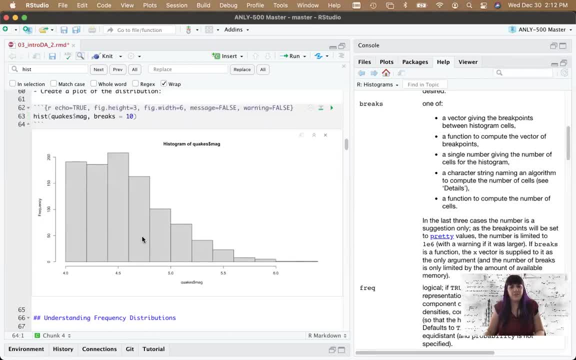 makes a lot more sense. one, two, three, four, five, six, seven, eight, nine, ten, huh, who knew um? so that's why you get one here for one. so it's not the width of the window, it's how many bars you are. i have to like call phone a friend here in a minute, okay, so 20. 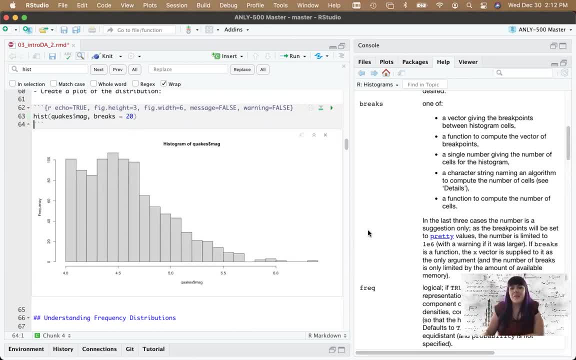 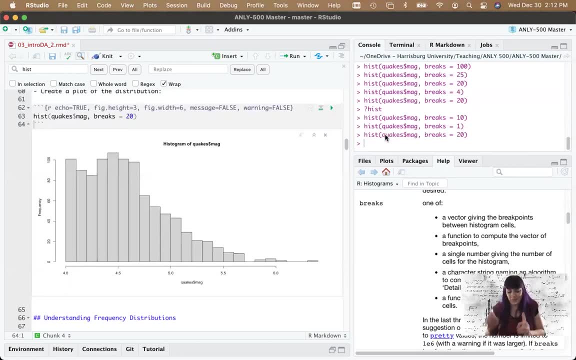 it's about 20 bars looks right for this, okay, um, or a function to compute the number of bars of cells? So here's why looking at the help is useful. So remember how to get there. question mark: name of the function, if I can type So again. I've always said that 15 magically is. 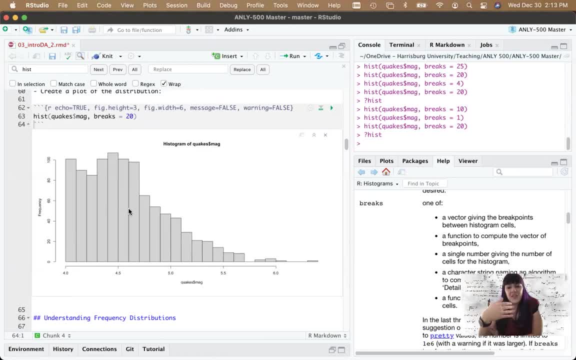 a really good number. It always seems to work really well for me, And that's probably because data representation wise, and the size that we're working with- somewhere between 15 to 20 bars- kind of makes sense. Now, on a one to seven scale, that number of bars makes no sense, right. So we 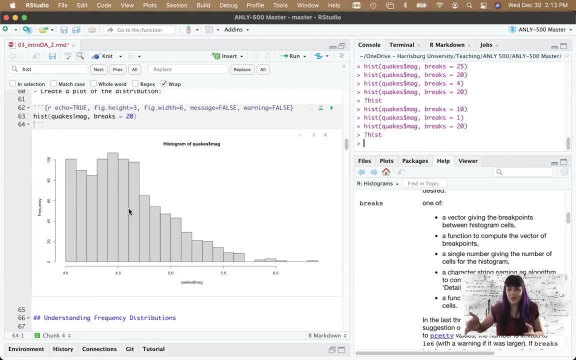 should probably think about seven, one for each point, Since we have a four to six scale in increments of 0.1.. So let's see, we've got 6.4 minus four, So 2.4 points divided by boop, boop, boop. 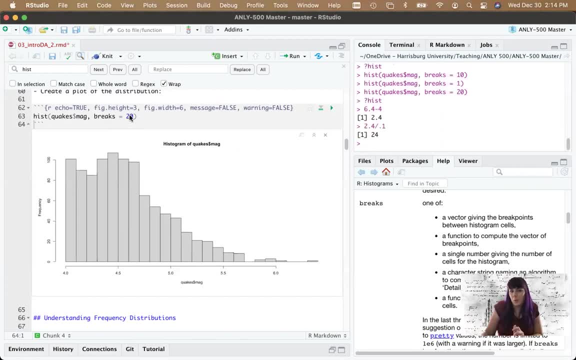 0.1 increments. So maybe 24 is the magic spot- possible numbers- And I didn't really change that much, okay, Because it's the number of possible points that could happen. Now, if we have a crazy number of decimals, we wouldn't want to do that, So just kind of play with it. Yeah, I'll leave it. 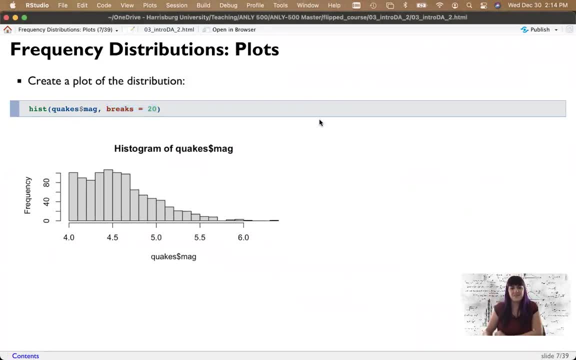 at 24.. I might put in what breaks means here in the notes too. right Now, what can I say about this graph? Well, Let's talk a little bit about how we describe these graphs. Yeah, So the properties of a frequency distribution. 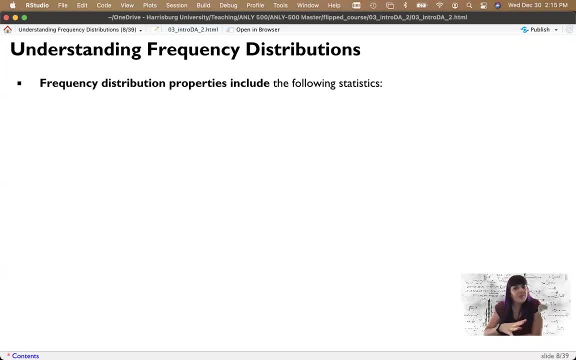 especially when we're comparing them to normal, include two kind of main descriptionuhrs. okay, So the first one is skew, and I've already kind of used that word, And this is the symmetry of the distribution. So we've talked about how the normal distribution 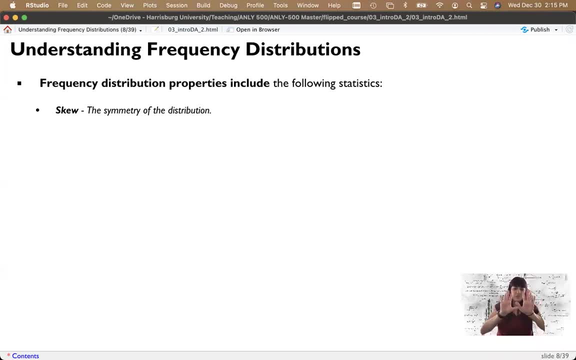 Hot dog fold, fold it and have it's the same on each side. If we cause that distribution to look weird, it NEW SC. 맛있 해주 SE لτο addition in zi lean right. it no longer folds correctly. i'm like trying to do this with my hands here, right? 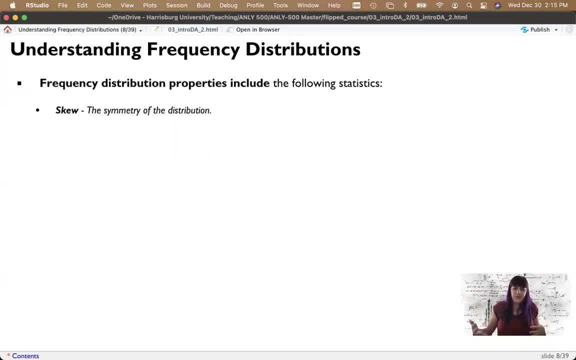 no longer folds correctly. so skew is how much it leans away from normal. this is a really easy political joke as well, right. so skews how much it leans to the left or how much it leans to the right. positive skew is where the scores are, are bunched at the low end and the tail points. 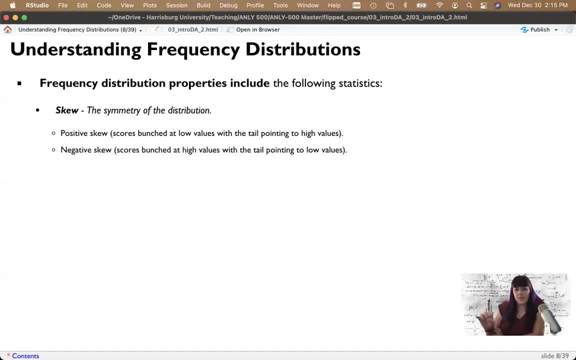 to the positive end. negative skews, where the scores are bunched to the high end, the tail points to the low end, and that always confuses the heck out of people, and what i would say is that what you need to know is that skew is where the data isn't okay, it's where the tail. 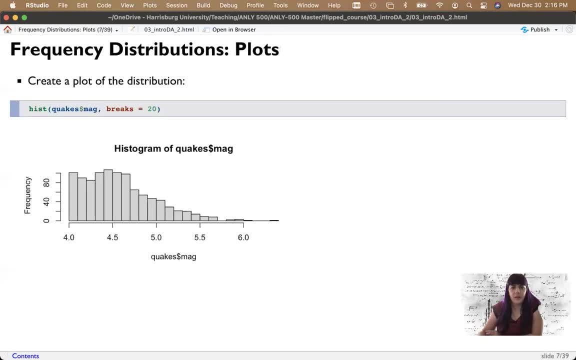 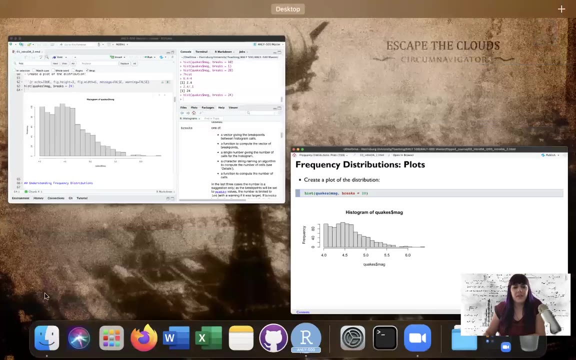 of the data is, and what i mean by tail, it's back up here here, so they're the tail of the data. so, to make this a perfect hot dog fold, we're missing all this data here on the right. okay, so this is a positive skew, even though it leans to the left. the other thing i've seen people do is: 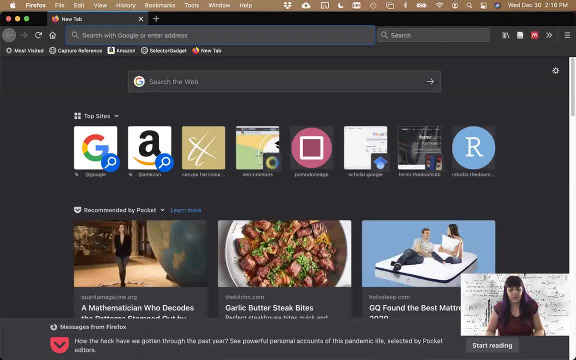 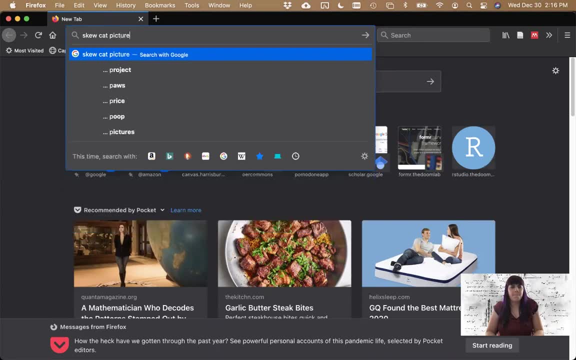 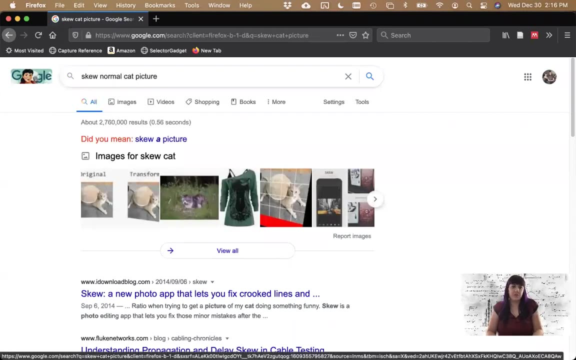 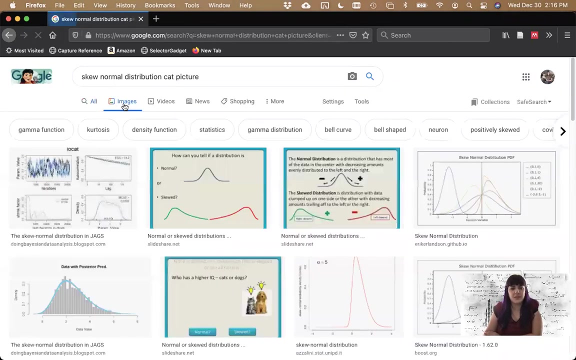 draw like cat ears on these so we can quick find a good google. don't let me down google. oh, i'm gonna get like pictures of cats, which is okay, i guess. yeah, i don't remember what textbook i got here. I saw this in where someone had drawn like a cat on the distribution. I can't draw, You don't. 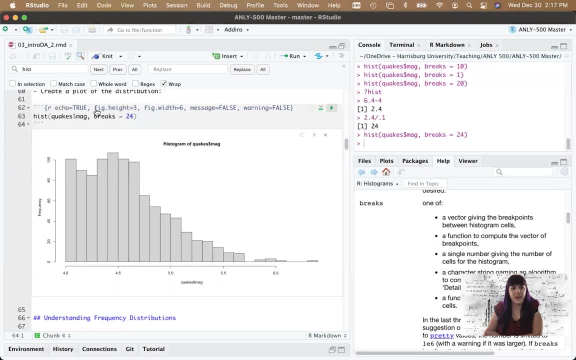 want to watch me do it, But basically the idea here is that you put the cat head here and the tail of the distribution is where the skew is. So you can remember that this is a little kitty cat and that tail over here indicates this is positive skew because the tail's on the positive 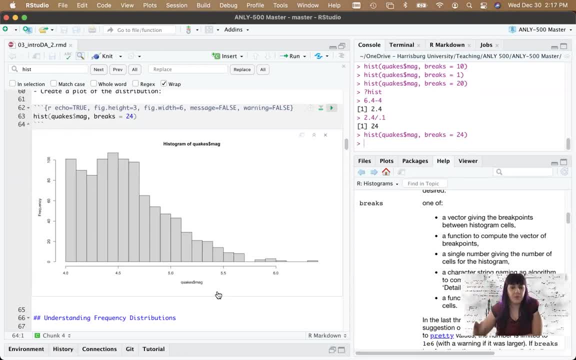 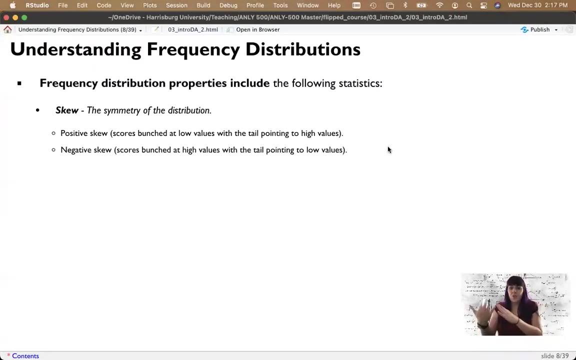 the higher side. Now, positive doesn't mean that the numbers physically are positive, because we don't have any negative numbers here. right, It runs from four to six. It just means that it's on the upper end of the graph. Negative skews the other way where the low values, even if they're 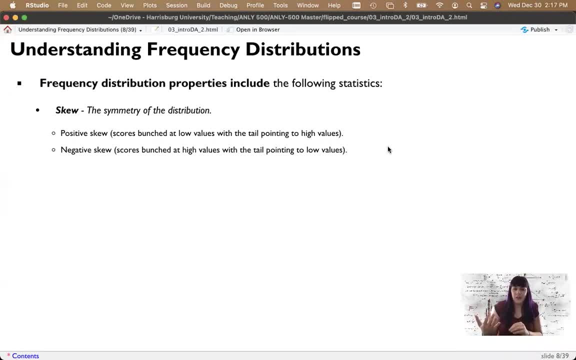 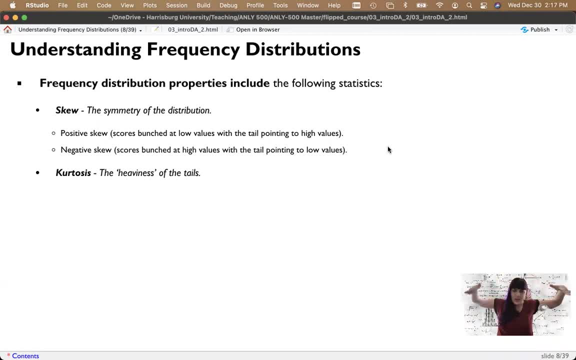 of the tails but that is determined by the spread of the data. So distribution that has been flattened out right. so you took a normal distribution and went squish and it's flattened out. we'll have what are called light tails. It's a platychartic distribution. 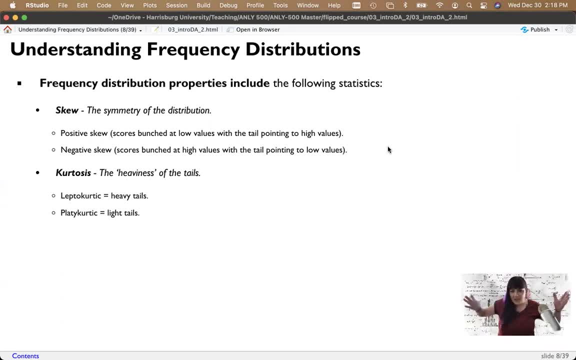 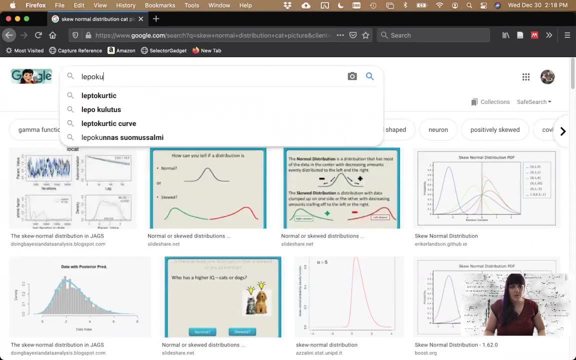 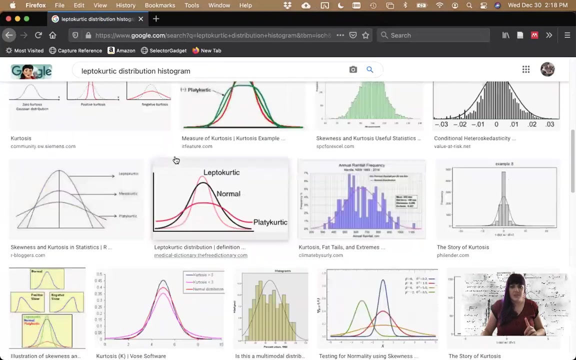 the second one here: A distribution that you've taken and go whoop squished in will have heavier tails. it's called a leptokurtic distribution and there's a very famous picture for these leptoker, very famous picture that i'm just gonna have to search the word here: kangaroo. 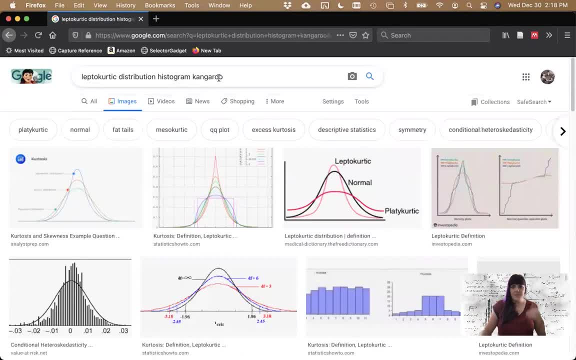 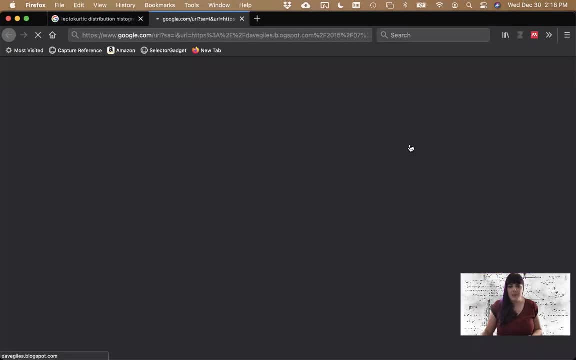 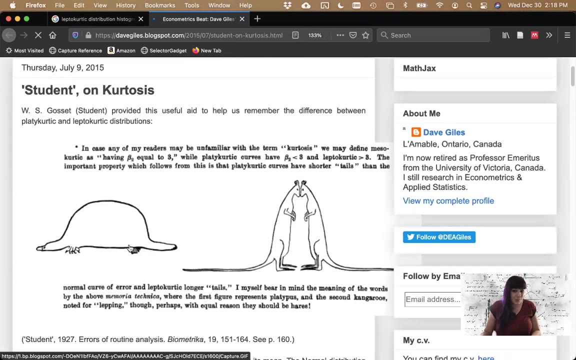 oh man, where's my platypus picture? ah, here, it is okay, so can i make it bigger? can i go to whatever this is? ah, so this is like super famous picture of a platycurtic distribution which is a platypus right, because it's flattened out from normal, and a leptokurtic distribution which is 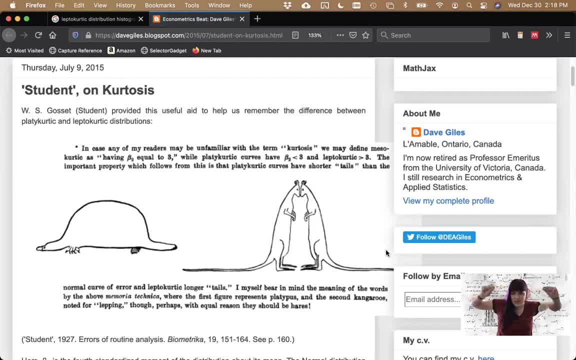 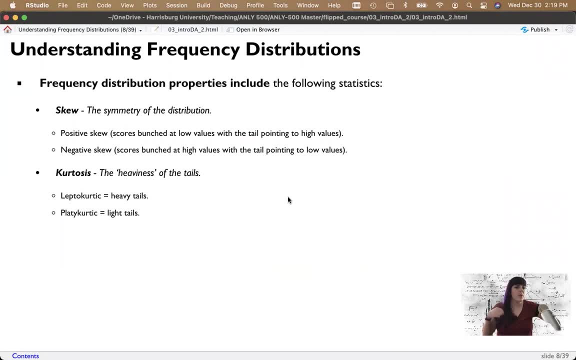 kangaroos, because they're fighting each other and they have long, skinny tails. okay, all right, so that's kurtosis, so that technically, the definition of kurtosis is based on the tails. but if you can remember platypus, flat, leptokurtic, kangaroo skinny, you'll be fine. 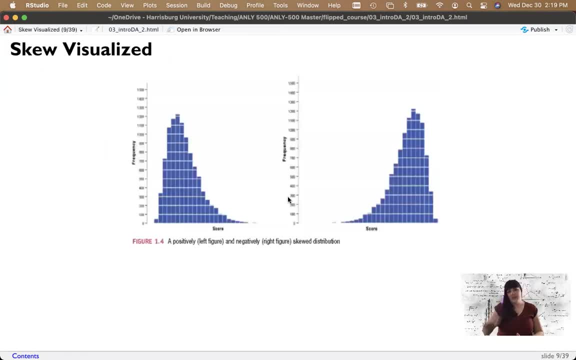 all right. so here's another picture of skew. so this one here would be a positive skew. so we've got a little cat head, the tails on the positive side. this one here would be negative skew because our tails on the negative all right. so here's another picture of skew. so this one here would be a positive skew. so we've got a little cat head the tails on the negative side. this one here would be a normal skew. so we've got a little cat head the tails on the negative side. this one here would be a normal su cables. okay, if you've got the lower side of the the graph. 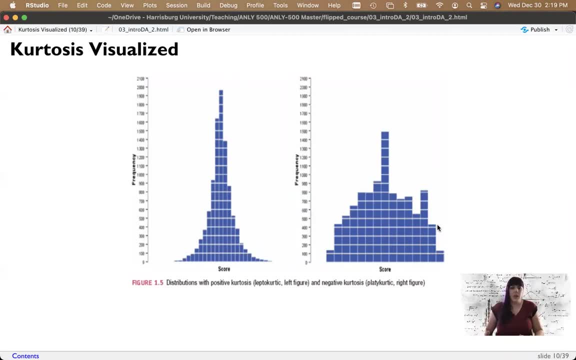 and here's an example of kurtosis, right? so this is a leptokurtic distribution, here a skinny distribution, and a platycurtic distribution, here a flatter distribution. okay, leptokurtic distributions are positive. okay, because they're skinnier than normal and um. 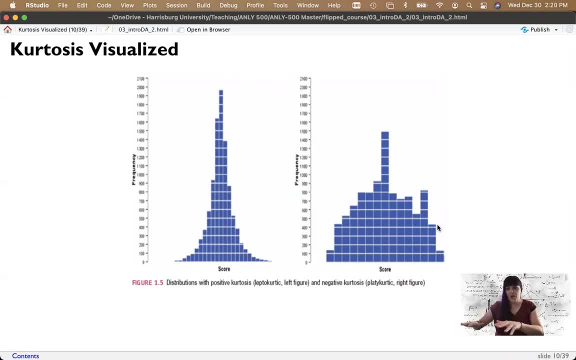 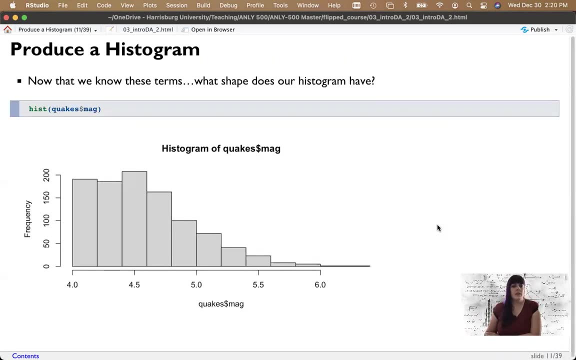 and platychartic distributions are negative when it comes to the numbers we're going to look at. So, now that we know these terms, what shape does our histogram have? And I didn't put any breaks in this one, so it will auto-pick a number of breaks for you, and that's approximately the. 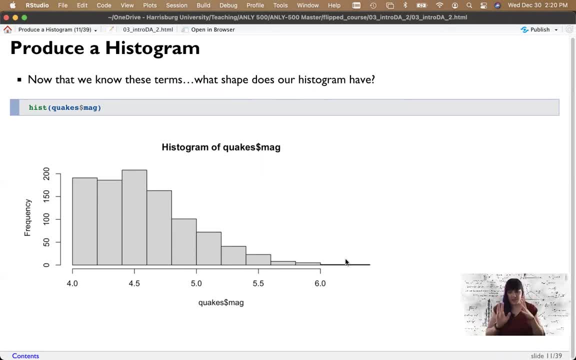 same kind of picture we've been looking at, even though we figured out that, like 20-24 breaks is the best Anywho. so it's definitely not normal. This is a skewed distribution, you know, towards the bottom. so it's positive skew because here's the tail And I'm not sure what I would think. 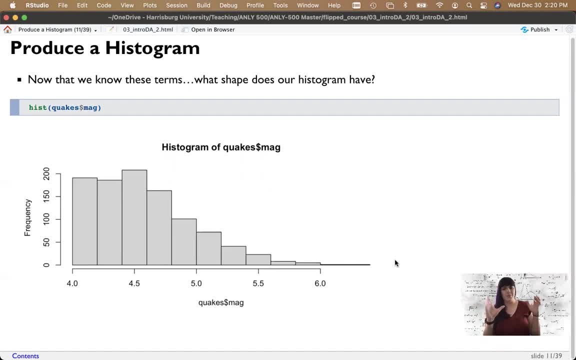 kurtosis-wise, because the skew is so, so strong. Well, it's not huge, but the skew is there, right? Maybe it's a little flattened from normal, okay, because it's a little more uniform, Uniform, meaning they have the same score as. 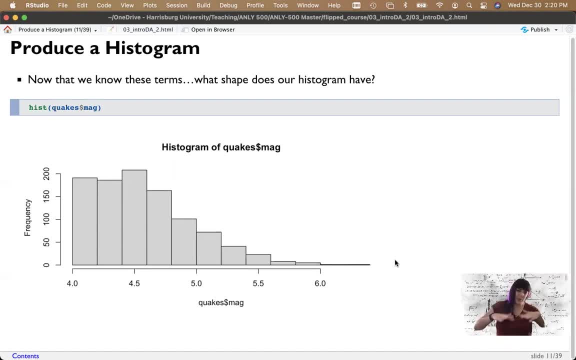 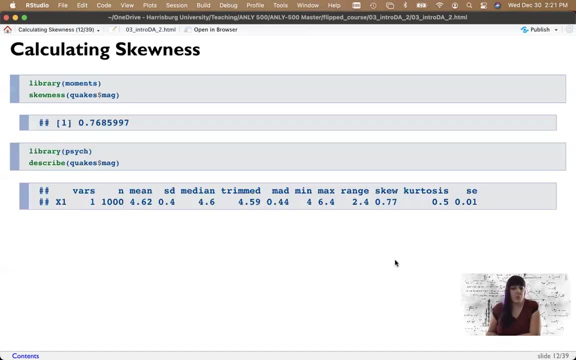 all the other ones All the way across. So maybe I would suggest that it's a little bit platychartic. okay, flatter than normal, Let's see. So there's a really cool package called moments. Now the moments package has two. 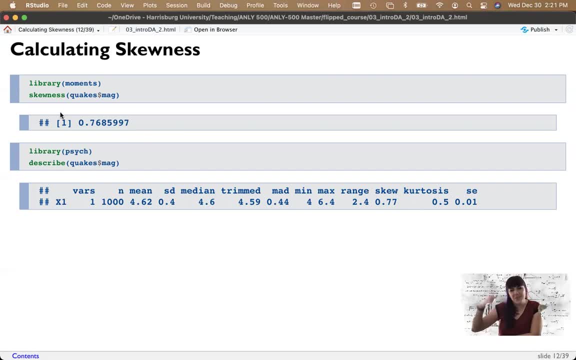 cool functions: skewness and kurtosis. Okay, it's not skew, it's skewness, And so you just put in the column that you're interested in, And so it tells us that the skew is positive. right, So it's 0.76.. We'll talk about how to interpret that in a second, Another cool package that you can look. 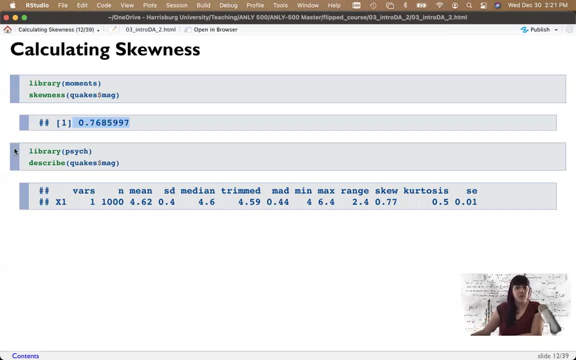 at is psych. We'll use the psych package a lot. It does a bunch of cool stuff And it gives you a bunch of statistics all at once. So I'll show this one over and over again. But it also tells us skew and kurtosis all at the same time. So I might bias you towards psych because it gives you so much. 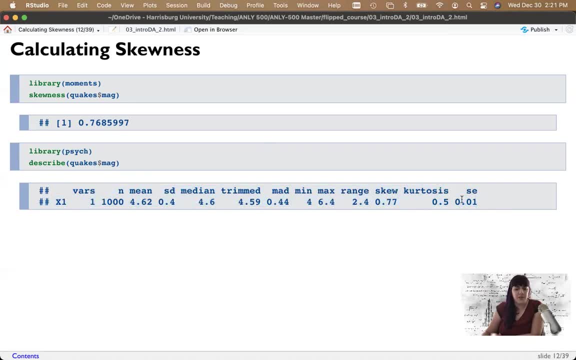 stuff, Even standard error, which we talked, which we have not talked about, sorry, which we're going to talk about, But it's a lot of stuff, So it's a lot of stuff, So it's a lot of stuff, So it's a lot of. 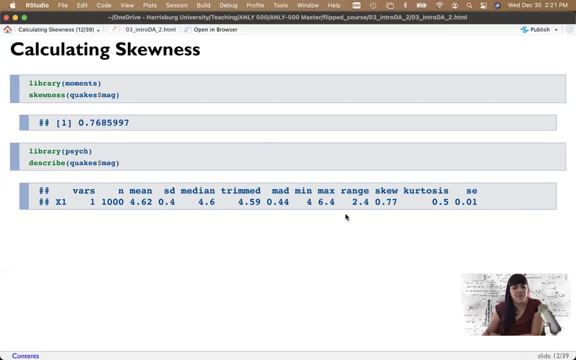 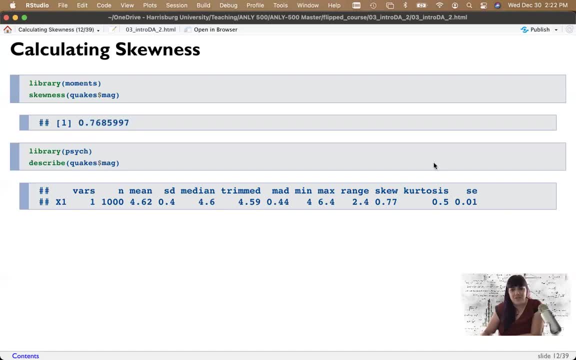 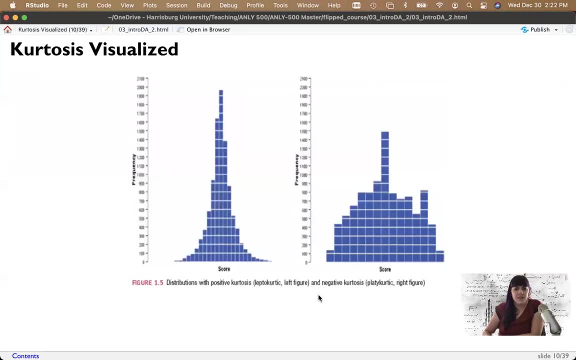 spend the time making the notes. We have not talked about standard error just yet, But it gives me skew and kurtosis at the same time. Now, what did we say? We said that leptokurtic distributions were positive. So I went through. I got it wrong. This is why the numbers are useful. 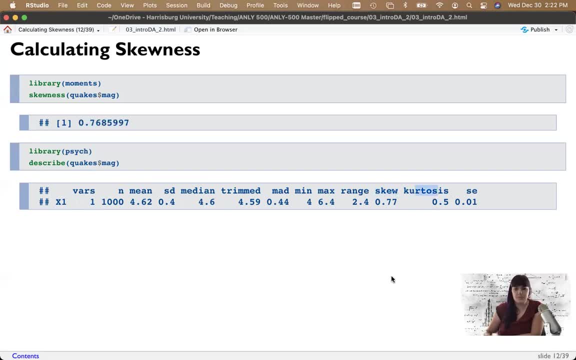 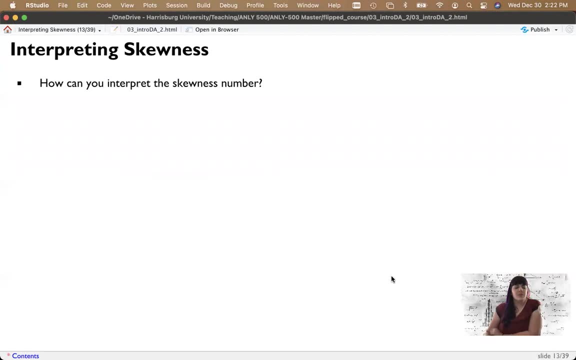 So skew is positive and so is kurtosis. Now you have to wait. there's a special interpretation for ketosis. So interpreting skewness here, how can we interpret this number? Well, there are ways to convert this number into a standardized value, but generally, 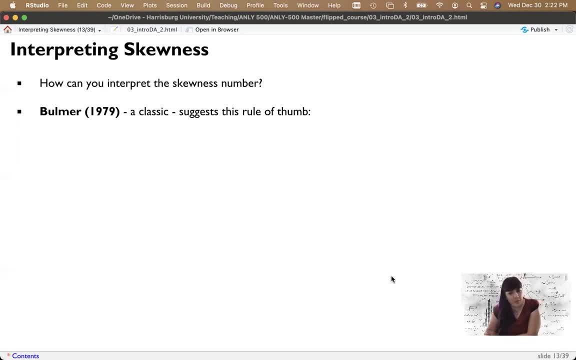 there are some rules of thumb here, and all semester we're going to talk about rules of thumb. There will be rules of thumb for nearly everything, but you have to remember that every rule of thumb is just that. It's just a suggestion. They're not hard and fast rules. 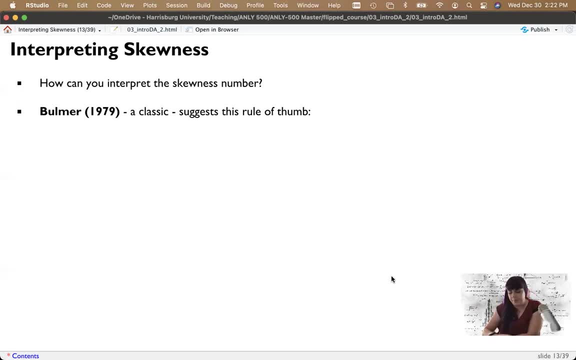 There are ways that we can kind of help us center our thinking. So if skewness is less than negative one or greater than one, so past one, the distribution is likely fairly skewed. Ours is 0.77, so okay, If the skewness is less than negative one, then the distribution is likely fairly skewed. 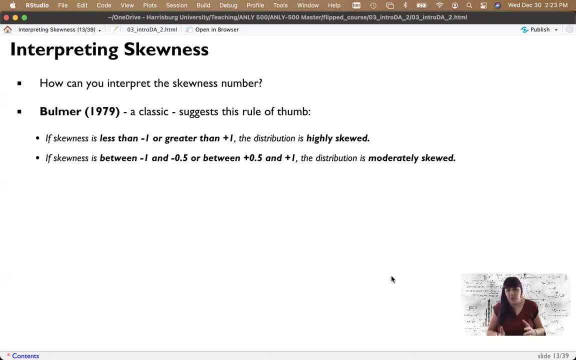 If the skewness is less than negative one, then the distribution is likely fairly skewed. If the skewness is between the absolute value of 0.5 and 1, it's moderately skewed. I'd say that's a good representation of the R graph. 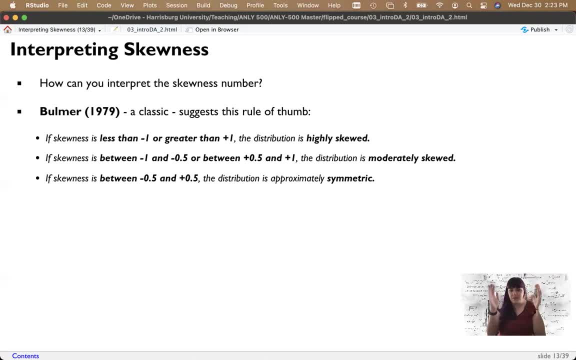 And if the skewness is between basically 0.5 and 0, then it's approximately symmetric. Okay, it may not be normal, but it's symmetric, so we can fold it in half. It may be symmetric and flat, so we can't say something is normal unless it's both symmetric and not. 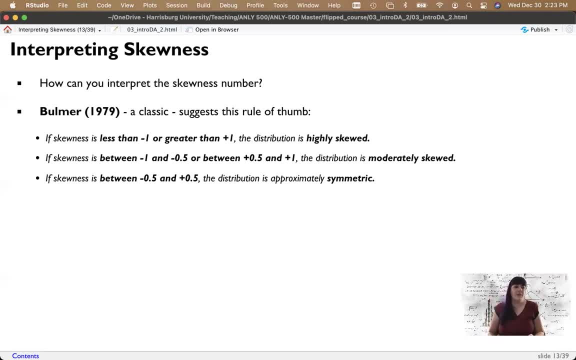 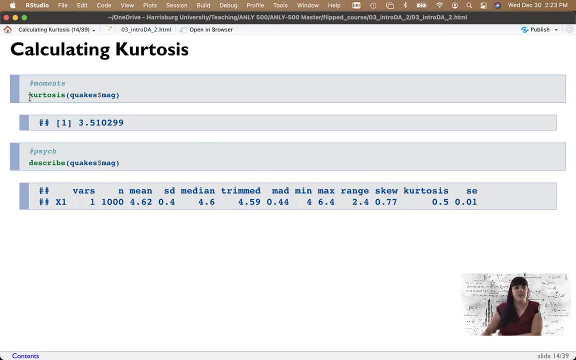 So R's falls in this moderately skewed category. Now with kurtosis, there's a function called kurtosis Okay. now I'm not sure. I think in the moments library it's not giving us the same type of kurtosis here. Obviously, these are pretty. 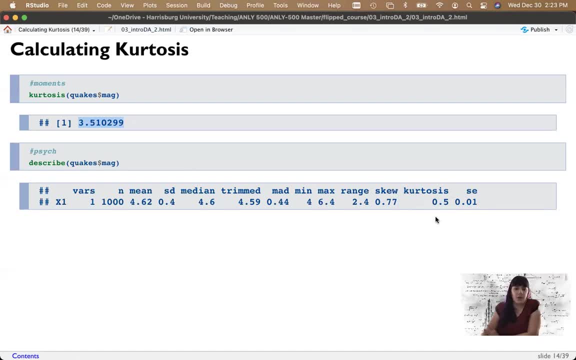 different. I think this one is giving us what's going to be called the excess kurtosis in psych and this one is giving us the literal kurtosis, which we'll get to in just a moment. But I think that's what we're going to do in just a second, but let's see if we can figure that out. 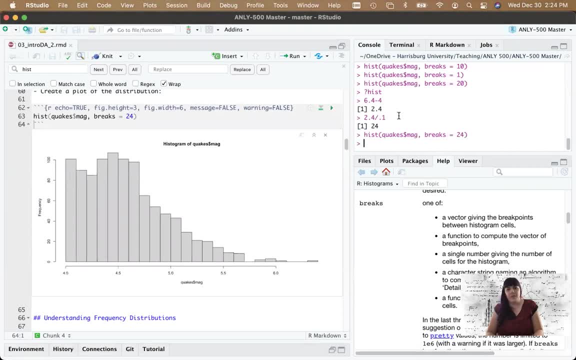 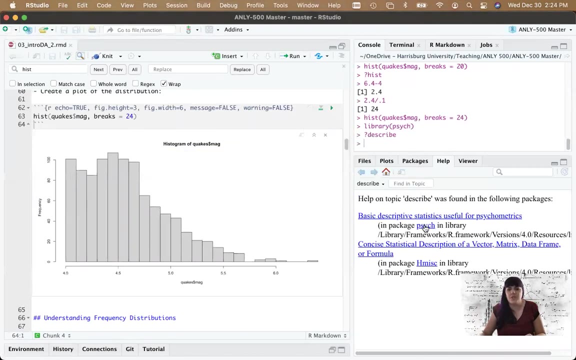 So we're going to Google, not Google, we're going to, I am, it is not even late, Like more coffee here, All right. so psych library: let's look at, describe which is a function in psych. here I want to describe. thank you. 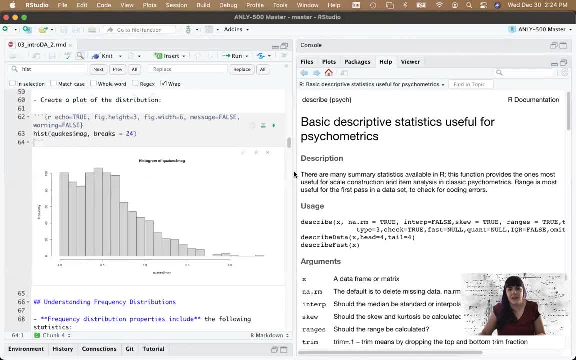 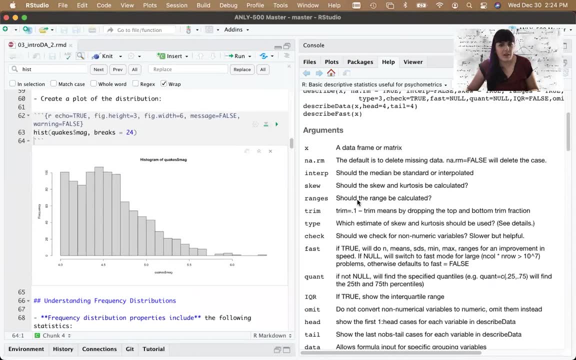 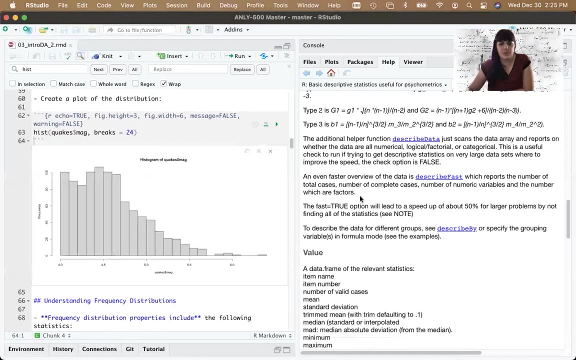 Okay, Now the great thing about the psych package is that it gives us just a whole bunch- I'm going to move my face up here real quick- of definitions of what it's calculating. So we're going to scroll, scroll, scroll. type one find skewedness and kurtosis. 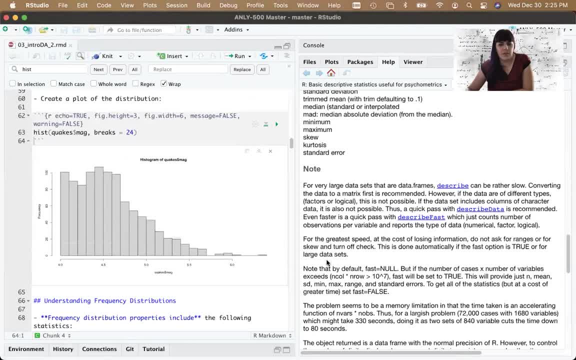 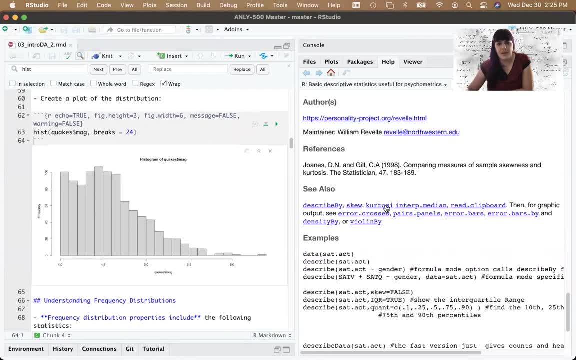 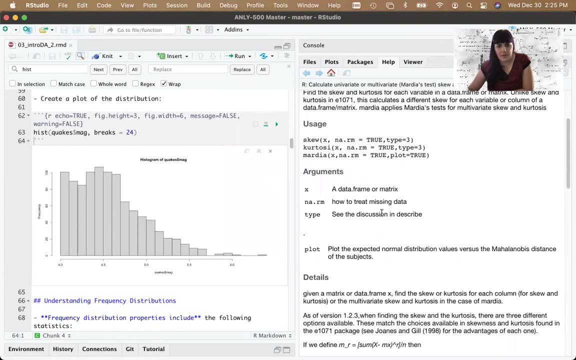 values skewed kurtosis. So I'm not gonna be able to find it quickly. My best guess is that it's giving us the kurtosis as the, as the as the excess kurtosis. Okay, And I will kind of comb through that and make sure that's correct. 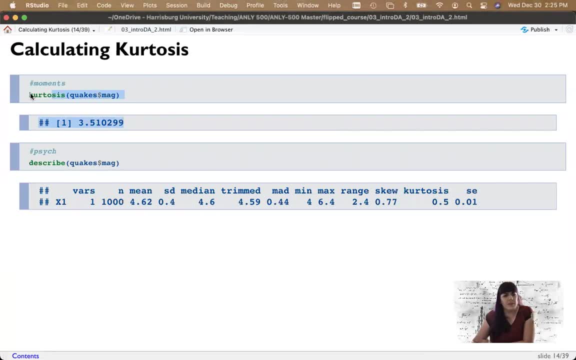 And how can I figure that out? Well, here, in moments, what we see is it gives us this 3.5. In psych, here it gives us 0.5.. Now, that seems pretty different, until I show you this slide. 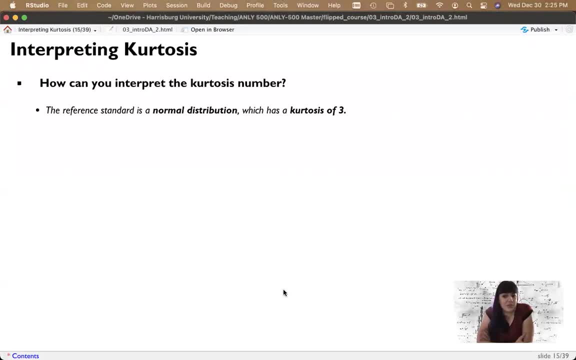 Where kurtosis actually, in a normal distribution, is three. Okay, So the default number, instead of being zero, is three. But to help with aid with interpretation, it's often what people often do is they subtract three from all the numbers. 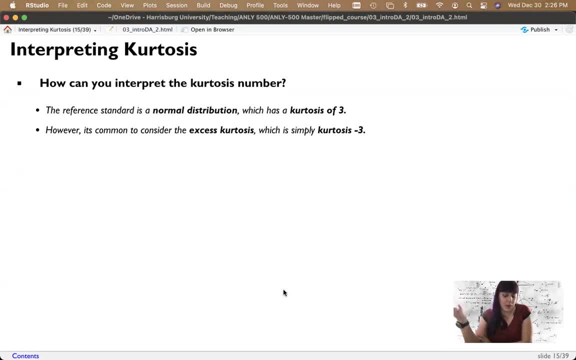 And so if we take our kurtosis value from moments, we 3.5 and we subtract three, we end up with the one in psych, which is 0.5.. So I think psych is giving you what's called excess kurtosis. 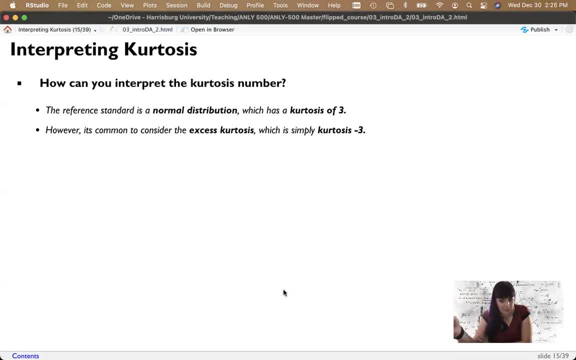 So how much more kurtotic kurtotic is it from normal? Okay, And so interpreting the excess kurtosis number can be done with. okay, So a normal distribution has a kurtosis of exactly three. Okay, So where the excess is zero, 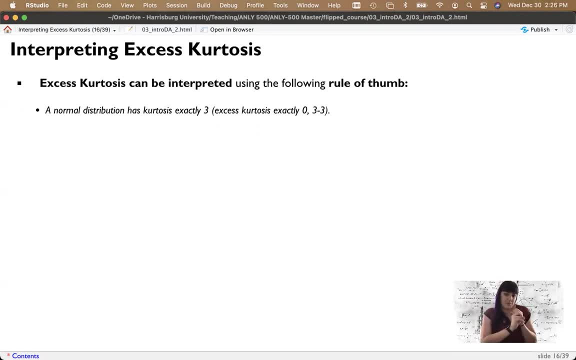 Okay. So if your kurtosis excess is zero from psych right, it's normal, Okay, It doesn't. it's not fat or skinny. It might skew. No, it's kind of it's hard to have distributions that are skewed. 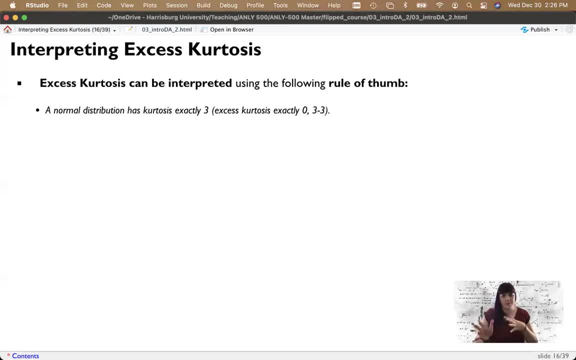 not also have kurtosis. So you can, you know, you can probably have a um, a non skewed distribution that has a lot of kurtosis, but it's hard when you skew things to keep it from getting skinnier fat. 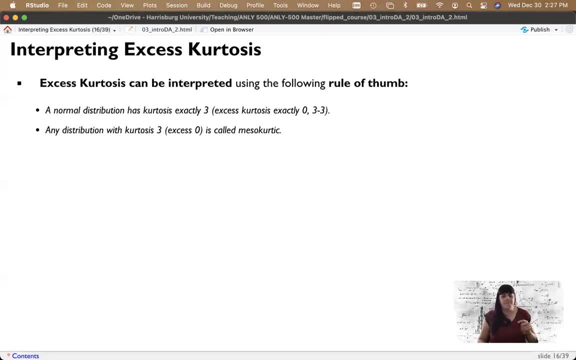 Now any distribution with um with a kurtosis at exactly three, so the excess is zero. that's called mesokurtic, Okay, Which just is a fancy word for normal Doesn't have kurtosis, Okay, So mesokurtic is normal. distributions with less than three. 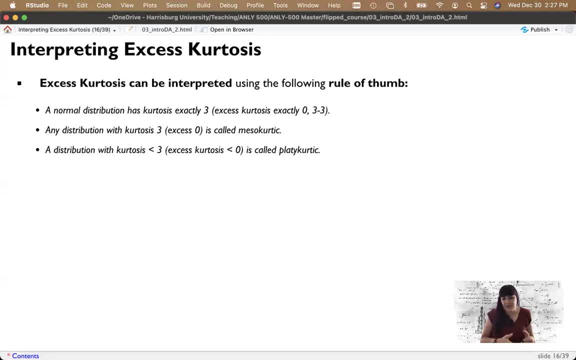 So this would be negative. kurtosis, excess kurtosis or platy kurtic, And that means that the tails are shorter and thinner. The central peak is lower. This is squished, Okay. Okay Distributions with an excess kurtosis. 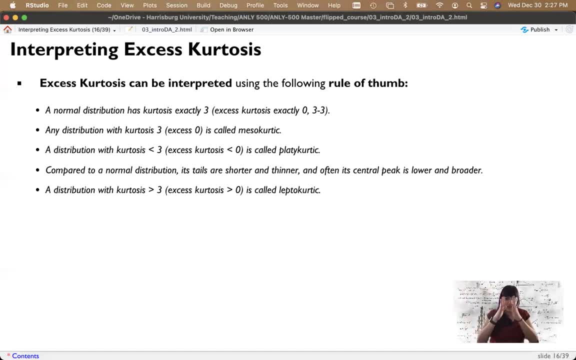 That's positive. So greater than three are leptokurtic. These are skinny kangaroo ones, And so the tails are longer and fatter, and this is often call uh, where the distribution is skinny. Okay, Now, I'm never going to like pop quiz. 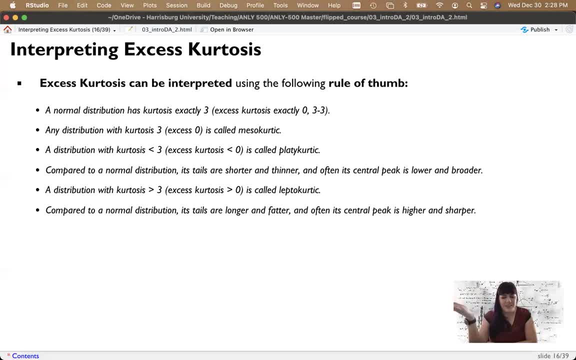 What's leptokurtic? right? You'll be able to look these up because it's easy to get them backwards, Uh, but you should be able to take a picture and look, calculate these numbers And use these rules to help yourself understand your distribution. 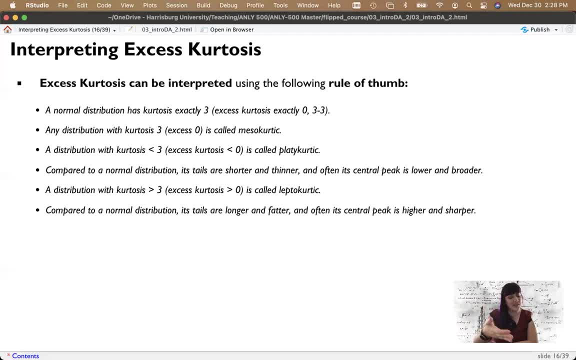 Okay, So we have as a moderately skewed distribution that has excess kurtosis. That's positive. Okay, So it's leptokurtic, And I mean, I've looked at these distributions for a long time and I, that graph, couldn't tell when I got it wrong. 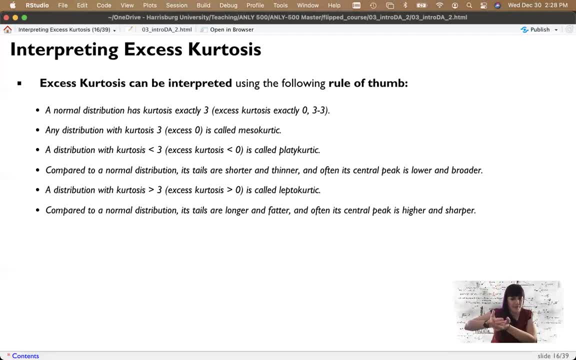 So be sure to use the numbers in tandem with the graph, And we'll talk a whole lot more about these. and why should you care, Should we be worried about that kind of stuff When we get to the data screening section? All right, 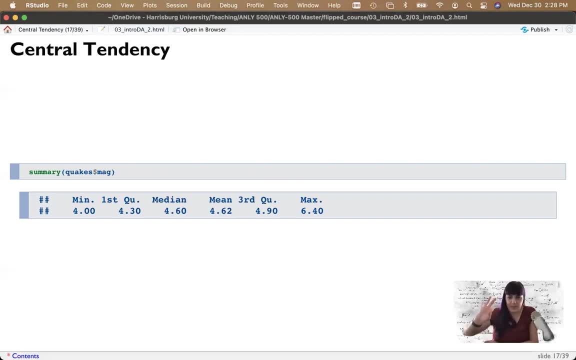 So let me see where was I going to stop. Okay, Couple more slides and then we'll break for this one and I'll have two videos. So we're going to switch here from frequency distributions to central tendency. Okay, So we went from. 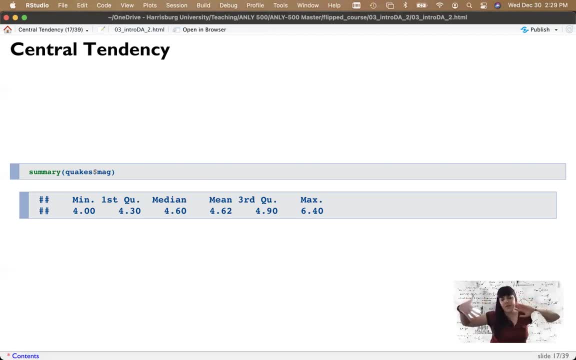 uh pictures right, Essentially to measures of, of distance. Now, central tendency is kind of the fancy name for where's the middle, And it's a single value that attempts to describe the data by identifying the middle. Okay, Now the middle can be defined in several ways. 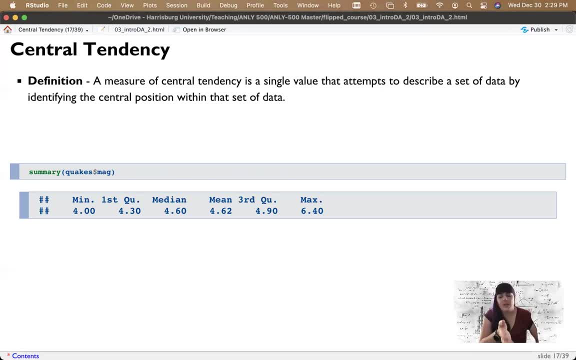 You wouldn't think this right, It's just the middle, And but what we can do is um, based on the type of distribution, define the middle a couple of ways. Okay, So measures of central tendency are sometimes called central location. 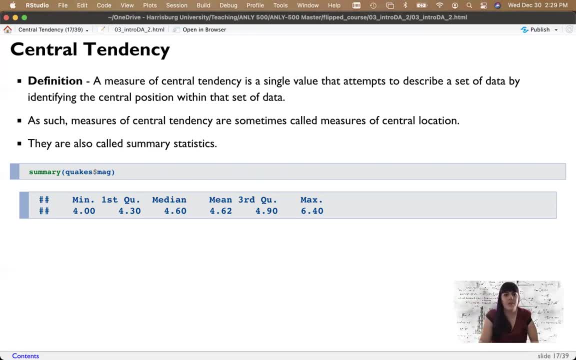 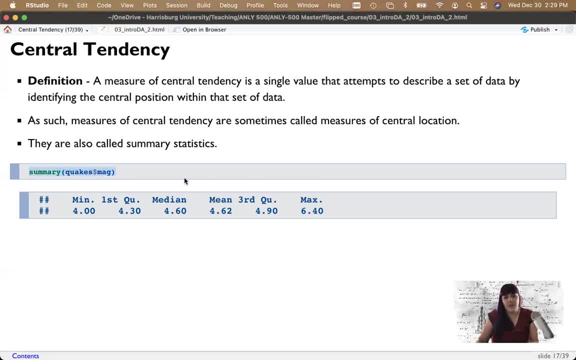 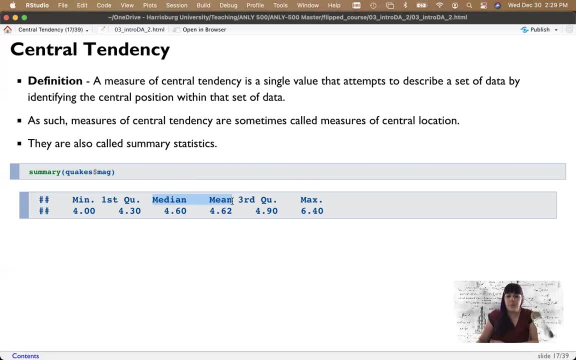 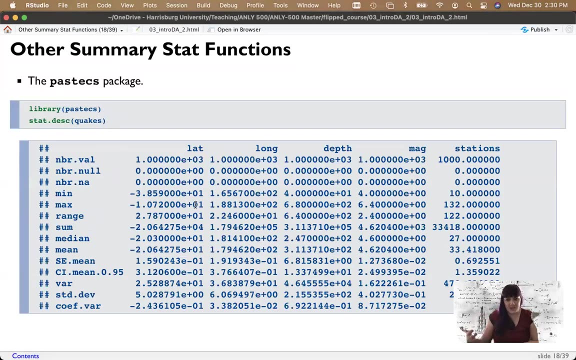 so the median skew is 4.6.. I'm sorry, The median magnitude of their earthquakes is 4.6 and the average is 4.62.. Pretty close. And then there are a couple of other packages here that i want to highlight. um, before we take a break in the paste cs package, okay now paste cs. 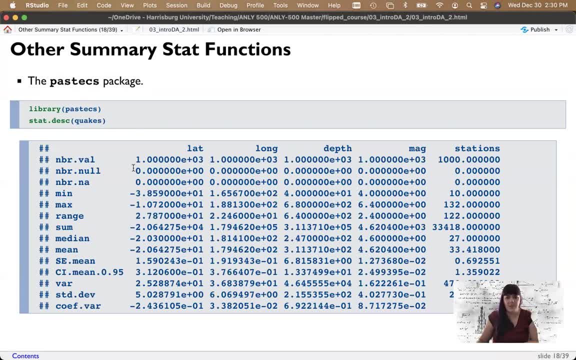 actually paste this in um in scientific notation, which we can turn off um. but the main thing that you want to be interested in here is it has the median and the mean, but it actually will allow you to calculate um on the whole. we calculated it on the whole data set. okay, you can actually do. 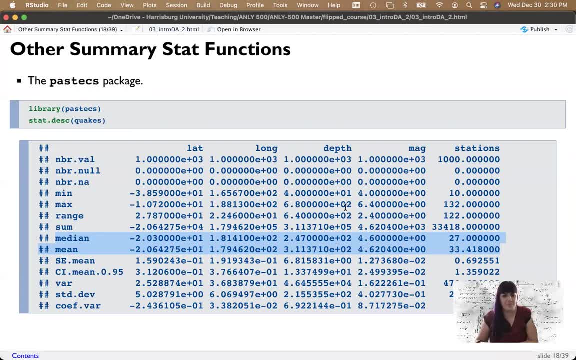 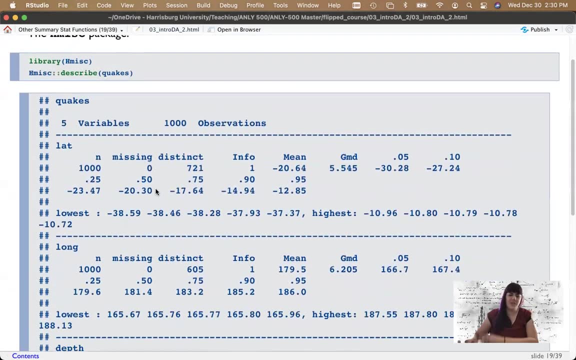 that with the summary function too, where we calculate on the whole data set. but also notice here it has got some other stuff that we were going to talk about. i said we're going to talk about later. h misc also has a few different ones. now i do love the output they. 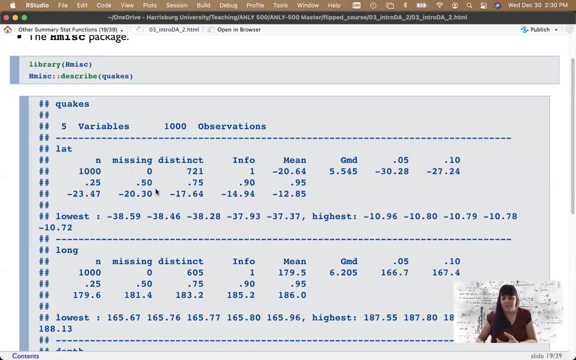 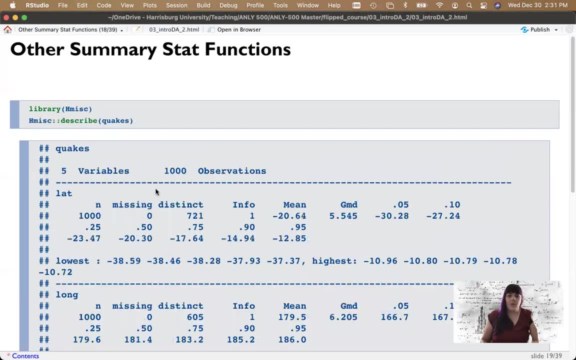 tried to make these kind of cutesy tables and that's great. but in the format here from paste cs, this is going to be easier for us to work with right. so when it prints out cute, it's hard sometimes to get it right. so when it prints out cute, it's hard sometimes to get it right. 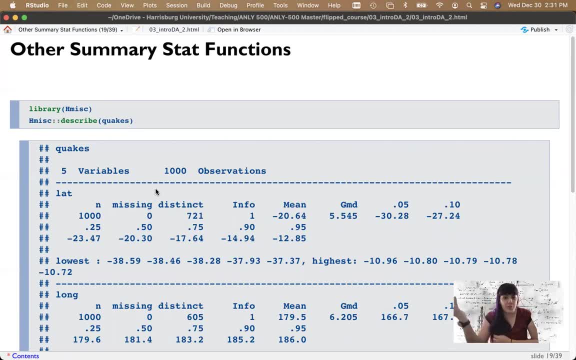 so when it prints out cute, it's hard sometimes to get it right. so when it prints out cute, it's hard sometimes to get the numbers into something a different formula or function, or to print them out. when it prints out in a table, it's easy to continue to manipulate and work with. 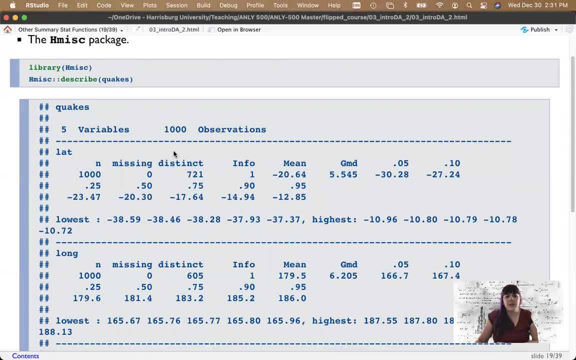 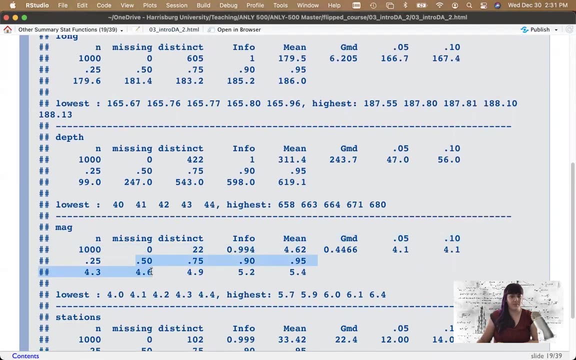 but you can pick your favorite one, um, so let's see where are we looking. here we've got the mean, and then the 0.5. here would be the median. okay, so let's look at the magnitudes to make sure that matches mean yes, and then 0.5. here is the median, and we'll talk about what. why is it 0.5? 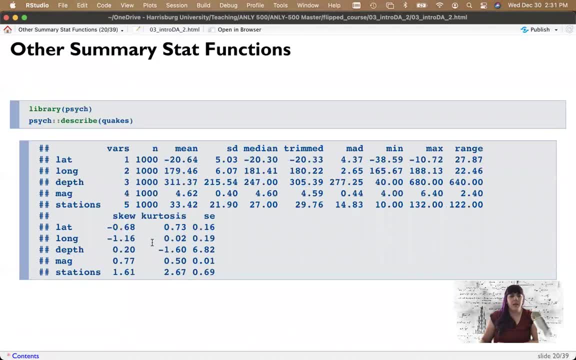 in the next lecture. all right, one last one and back to psych. so psych's describe function will actually take the entire data frame and describe it for you. it's really great if it's a character value. it just basically just says like i, i can't do this, don't ask me to um, but it will give you.